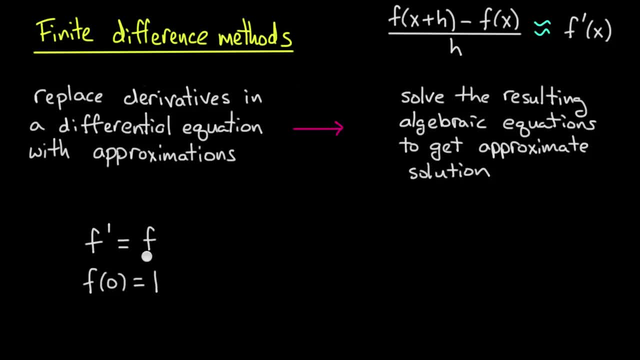 So here's a differential equation that we're familiar with: f' equals f. with an initial condition: f equals 1.. So you know how to solve this. The solution is to use the differential equation: f of x equals e to the x. The solution to this differential equation would be f. 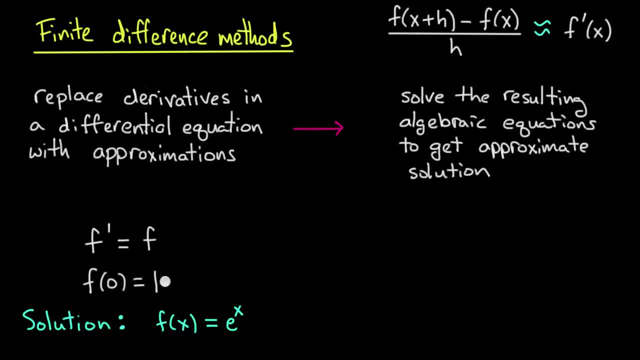 of x equals some constant times e to the x, and the initial condition would fix that constant at 1.. So let's see if we can replace the derivative here in this differential equation with a difference quotient approximation and see what happens. I take the f prime and I replace it with f of x plus h minus f of x. 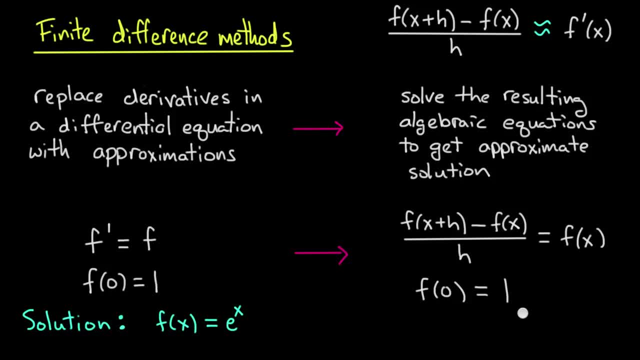 divided by h, and I keep that same initial condition. So here are my finite difference equations. Now let me rewrite this first equation just slightly so it's a little more suggestive as to how we're going to solve it. So I'll multiply both sides by h and add my f of x and it turns into f of x plus h equals. 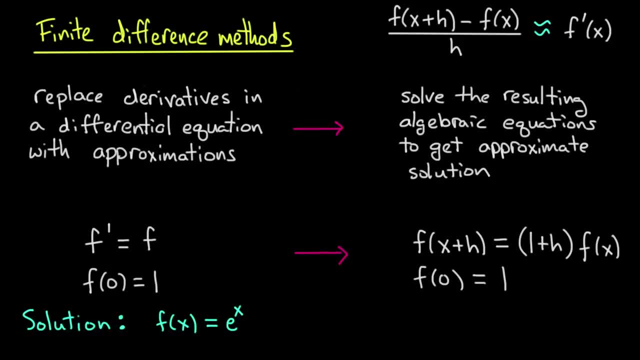 1 plus h times f of x. Notice now that we can solve the equation incrementally. We can start at f of 0 equals 1, and then we can use this finite difference equation to get the value at f plus h and then f plus. 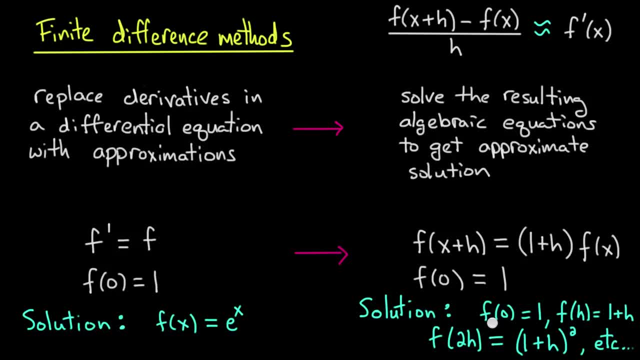 h, etc. So we get a solution which is f equals 1, f is 1 plus h, that's 1 plus h times f. f is 1 plus h times f, so that's 1 plus h squared, etc. And so we would. 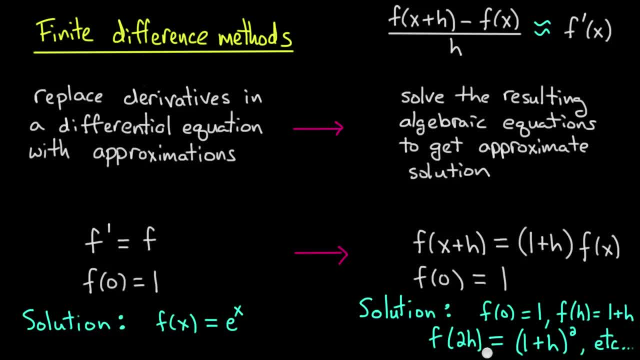 have 1 plus, say, k times h equals 1 plus h to the k. Now you might be satisfied with that, but I'm not, and the reason is there's a conflict of notation. We're using f to denote our actual solution over here, and over here we're using f, f, f, etc. 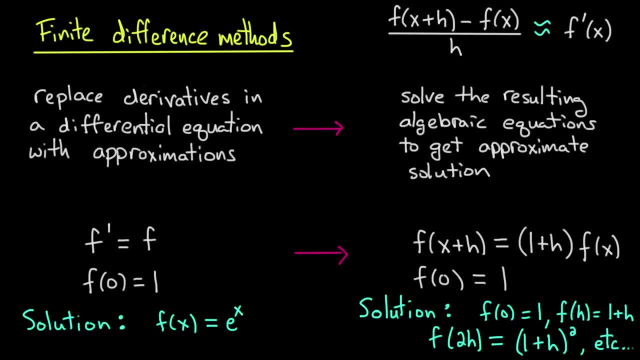 to denote the approximation to the actual solution. It's not true that f equals e to the h. It's only an approximation. 1 plus h is approximately equal to e to the h. So here's what we'll do. instead, We're. 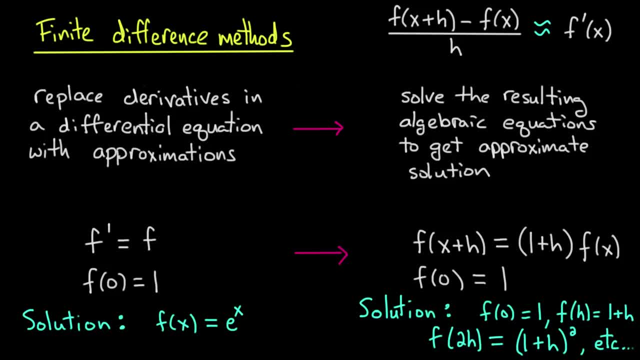 looking to approximate the function f at the points 0 and h and 2h, etc. So instead of calling those approximate values f, f, etc. we'll call them fk. and fk will be an approximation to f at the point xk, where xk is k times h. Now the sequence fk. 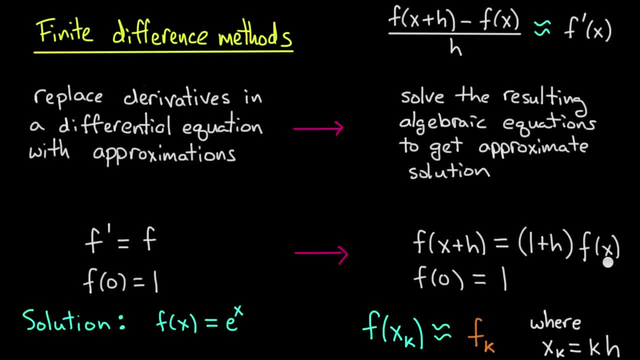 k will be defined by the finite difference equation above. Just like we found f of x plus h, knowing what f of x is, we'll define a sequence where we determine f of k plus 1, knowing what f k is, in the exact same formula. So we start off at f0, you plug in f0, you. 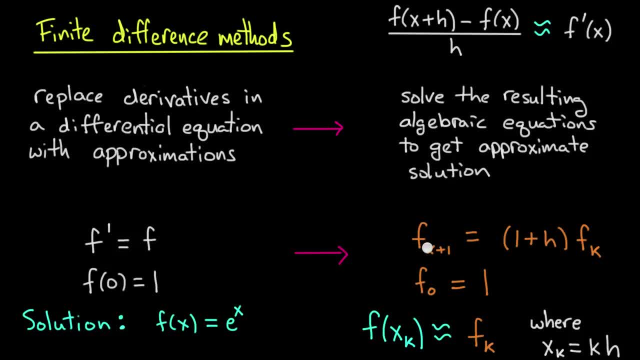 find out what f1 is, you plug in f1, you find out what f2 is, etc. And the hope is that that sequence will approximate the real solution, f, at the points that we can access by incrementing h. In other words, xk equals k times h. 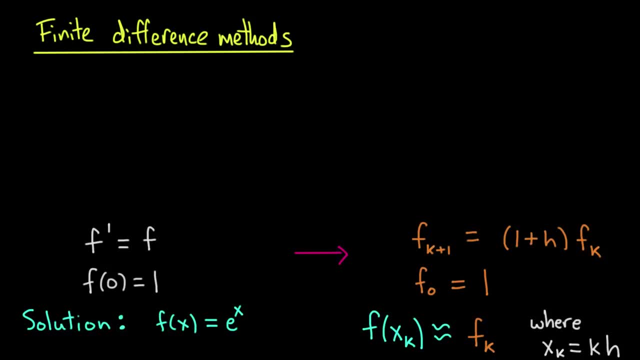 I'd like to conclude with a concrete computation for a particular value of h. Let's choose: h equals 0.5.. Now I start out with f0 equals 1.. I plug that in to get f1.. I plug in f0. 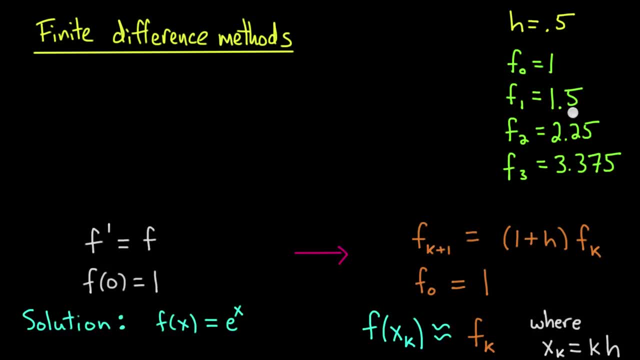 equals 1,. I have 1 plus 0.5 times 1, and that's 1.5.. I plug in f1 to get f2.. Put in 1.5 for f1.. 0.5.. 0.5.. 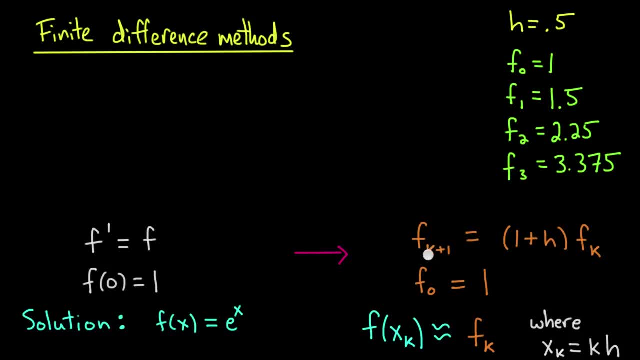 0.5. 0.5. 0.5. 0.5.. That's 1.5 times 1.5.. And I get f2, which is 2.25, etc. Now I can plot those guys roughly on a graph. What I've done here is I've got my x axis. 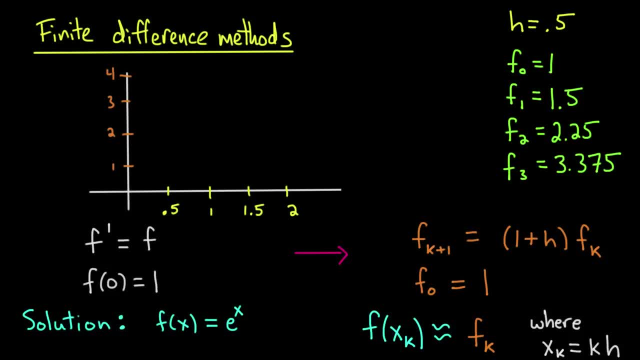 and the axis, which is where I'm going to plot f of x. I get various values. This is f0, which is 1.. This is f1, which is 1.5.. This is f2, which is 2.25.. And this is f3, which is 3.370,. 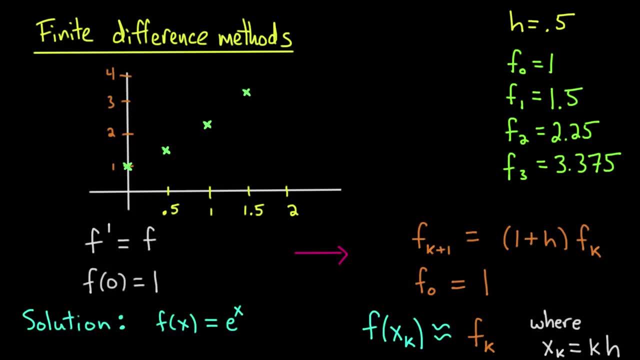 3.375.. Now you can compare that with the values of the actual solution. since we know the actual solution, it's e to the x. The actual solution evaluated at 0 is 1.. The actual solution evaluated at 0.5 is approximately 1.65, so that's a little over my approximation of 1.5.